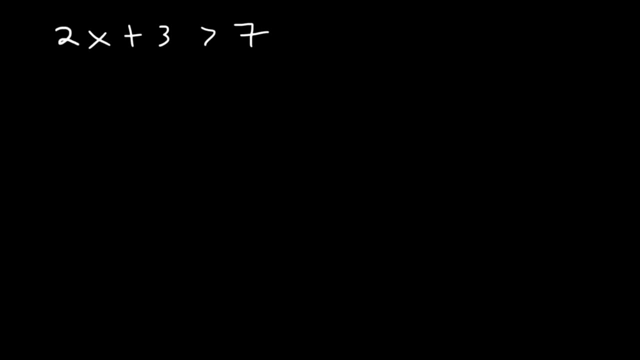 You can treat the greatest sign as if it's an equal sign. The only difference is when you have the solution, you should plot it on a number line. So let's begin by subtracting both sides by 3.. These will cancel, And so 2x is greater than 7 minus 3, which is 4.. 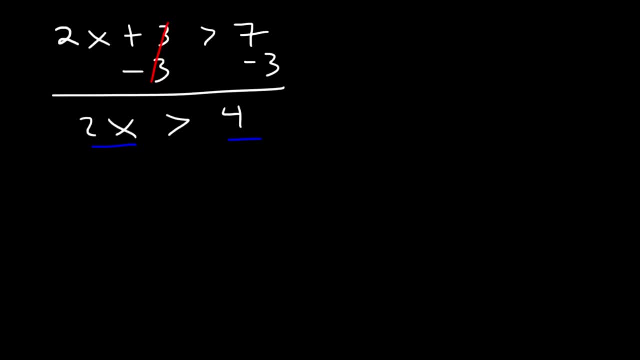 Next, let's divide both sides by 2.. And so we can see that x is greater than 4 divided by 2, which is 2.. And now let's plot it on a number line, So here's 2.. Because it's greater than but not equal to. we're going to have an open circle. 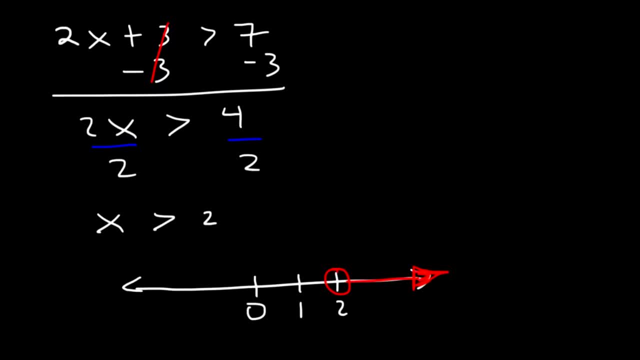 And since it's greater than we're going to shade towards the right, That is, towards positive infinity. So to represent the answer using interval notation, it's from 2 to infinity. Now let's try another example. Try this one. 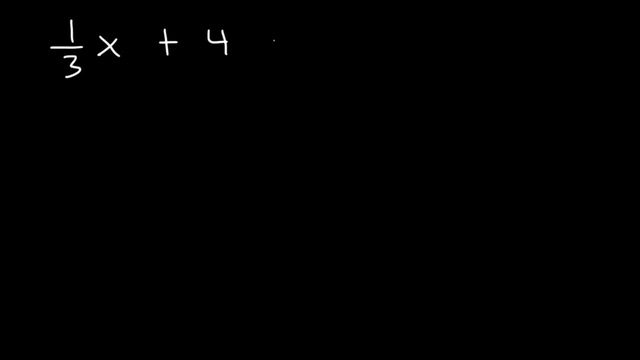 1 third x plus 4 is less than or equal to 6.. Feel free to pause the video and work on this example. Now. let's begin by subtracting 4 from both sides. So 1 third x is less than or equal to 6 minus 4, which is 2.. 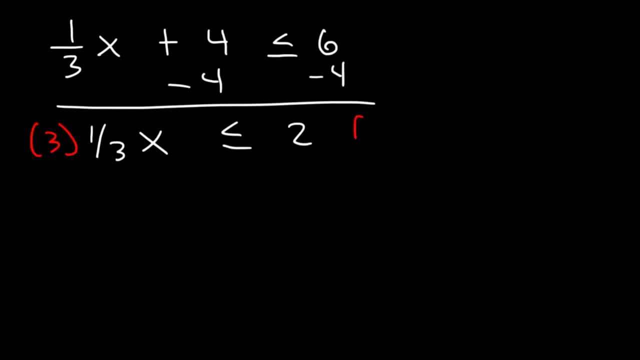 Next, let's get rid of the fractions. So let's multiply both sides by 3.. 3 times 1, third is 1.. So we're going to be left with 1x or just x. 2 times 3 is 6.. 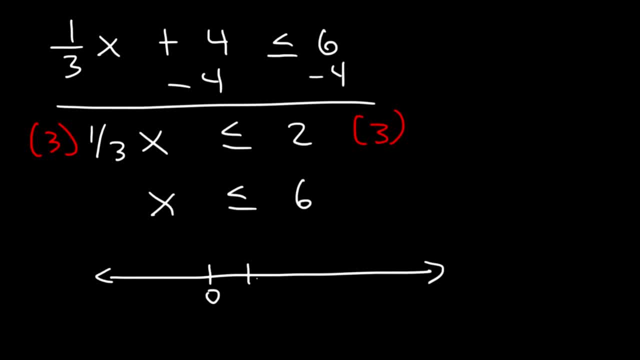 So x is less than or equal to 6.. So this time we're going to have a closed circle And because it's less than, we're going to shade towards the left, That is, towards negative infinity. So to represent the answer using interval notation, it's from negative infinity to 6.. 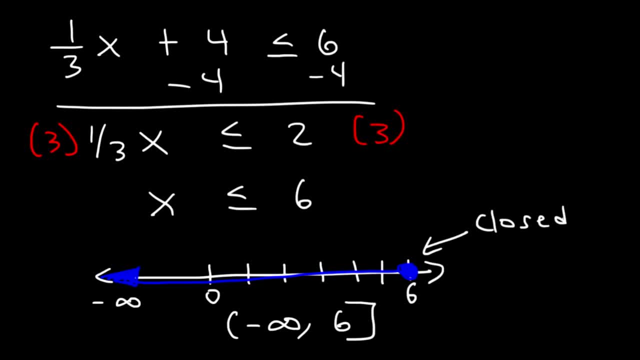 But because we have a closed circle at 6, we're going to use brackets, But keep in mind you should always have parentheses any time you're dealing with infinity. Let's try another example. Go ahead and find the solution to this equation. 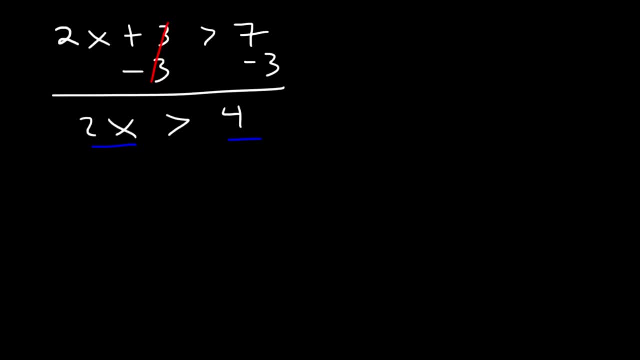 Next, let's divide both sides by 2.. And so we can see that x is greater than 4 divided by 2, which is 2.. And now let's plot it on a number line, So here's 2.. Because it's greater than but not equal to. we're going to have an open circle. 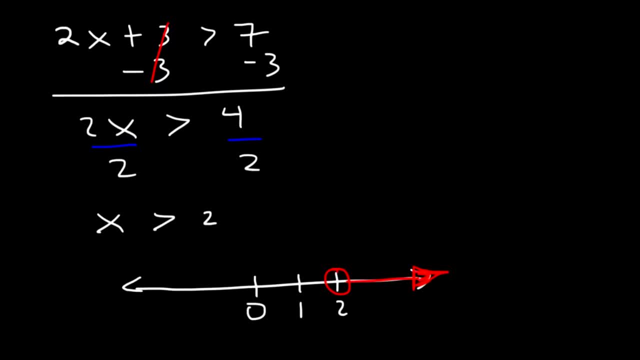 And since it's greater than we're going to shade towards the right, That is, towards positive infinity. So to represent the answer using interval notation, it's from 2 to infinity. Now let's try another example. Try this one. 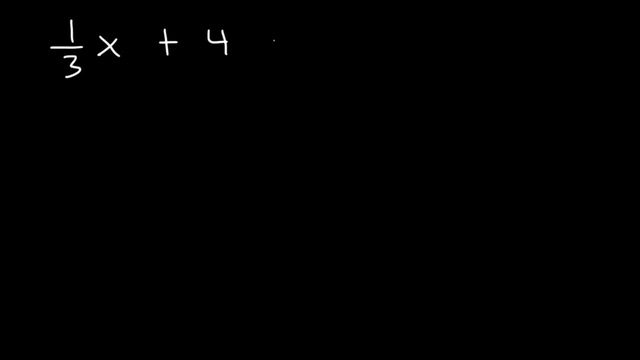 1 third x plus 4 is less than or equal to 6.. Feel free to pause the video and work on this example. Now. let's begin by subtracting 4 from both sides. So 1 third x is less than or equal to 6 minus 4, which is 2.. 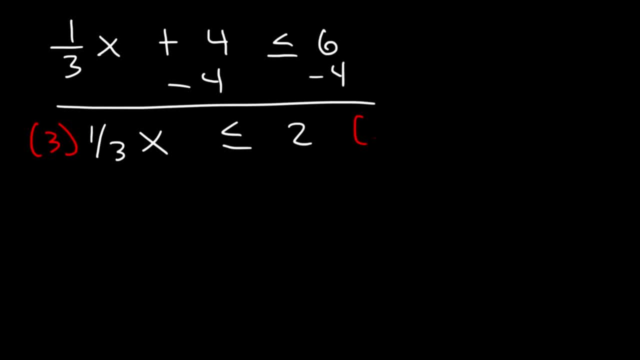 Next, let's get rid of the fractions. So let's multiply both sides by 3.. 3 times 1, third is 1.. So we're going to be left with 1x or just x. 2 times 3 is 6.. 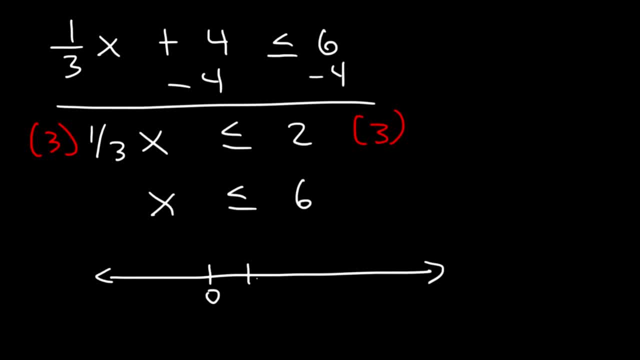 So x is less than or equal to 6.. So this time we're going to have a closed circle And because it's less than, we're going to shade towards the left, That is, towards negative infinity. So to represent the answer using interval notation, it's from negative infinity to 6.. 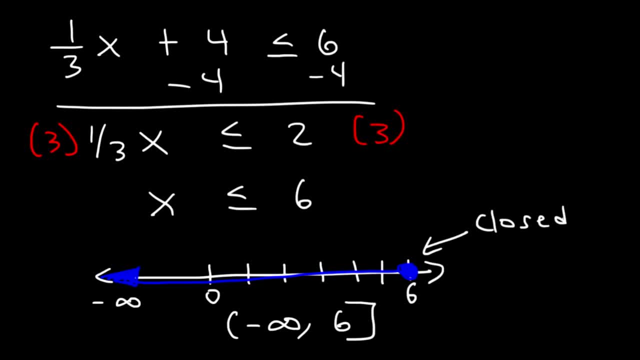 But because we have a closed circle at 6, we're going to use brackets, But keep in mind you should always have parentheses any time you're dealing with infinity. Let's try another example. Go ahead and find the solution to this equation. 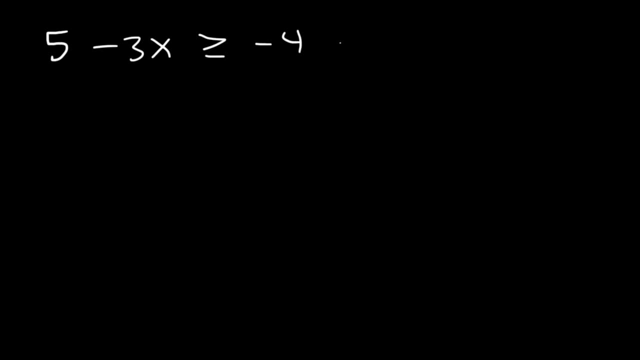 And then plot it on a number line. So what do you think the first thing we should do in this example? Should we divide by negative 3 or subtract by 5? What you want to do is subtract by 5 first. These will cancel. 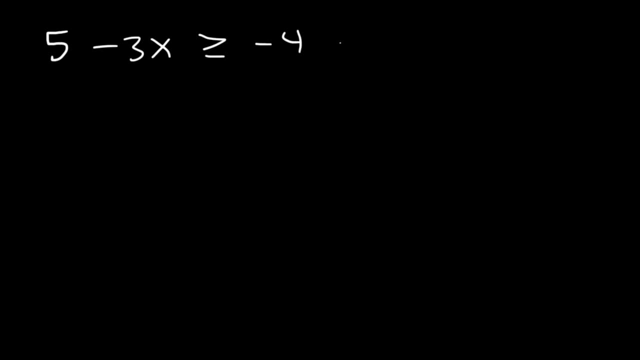 And then plot it on a number line. So what do you think the first thing we should do in this example? Should we divide by negative 3 or subtract by 5? What you want to do is subtract by 5 first. These will cancel. 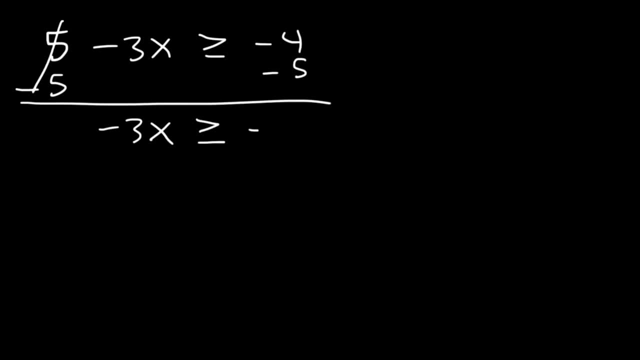 Negative 3x will be equal to or greater than negative 4 minus 5,, which is negative 9.. Next, we need to divide both sides by negative 3.. Now here's a question for you: When you divide or multiply by a negative number, does anything special happen? 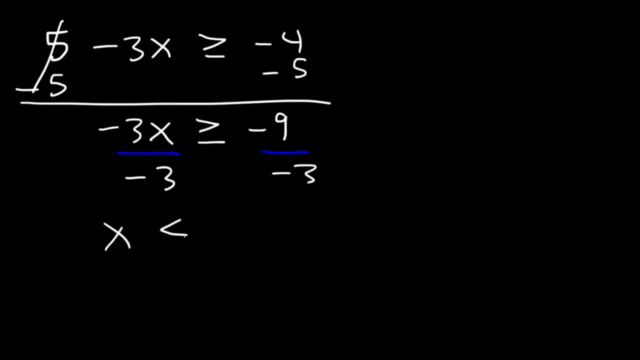 And the answer is yes. When you multiply or divide by a negative number, you need to change the direction of the inequality sign. Negative 9 divided by negative 3 is positive 3.. And now we can plot the solution on a number line. 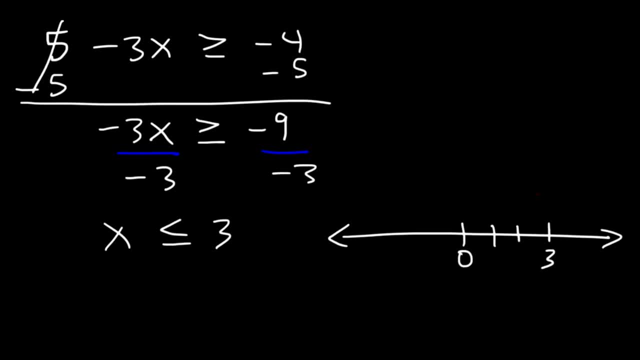 So X is less than or equal to 3.. So we're going to have a closed circle shaded towards the left because it's less than So. the solution using interval notation is negative infinity: negative infinity to 3 using brackets. here's the next one. let's say: if we have 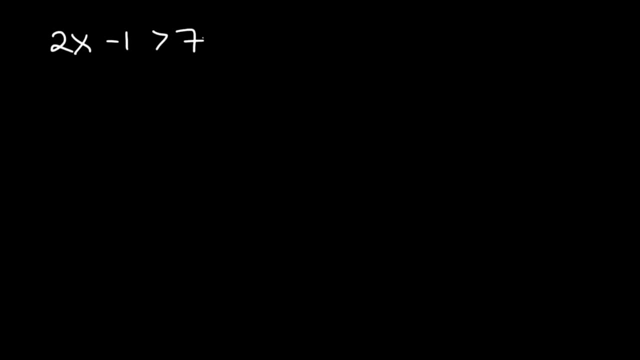 2x minus 1 is greater than 7 or negative. 3x plus 2 is equal to or greater than negative 1. solve the equations. so let's start with the first one. let's add 1 to both sides, so 2x is greater than 8. next let's divide both sides by 2. 8 divided. 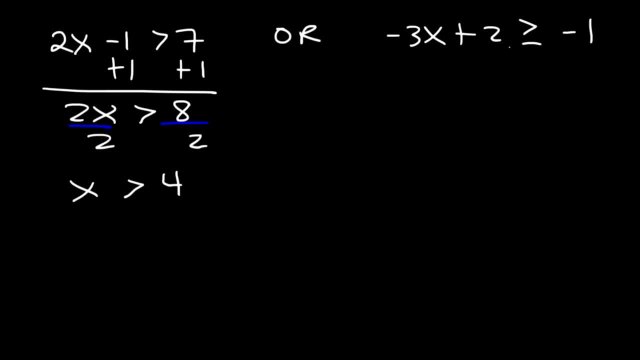 by 2 is 4, so X is greater than 4. now, before we plot on the number line, let's solve the other one. let's subtract both sides by 2. negative 1 minus 2 is negative 3. next, let's divide by negative 3. don't forget to change the direction. 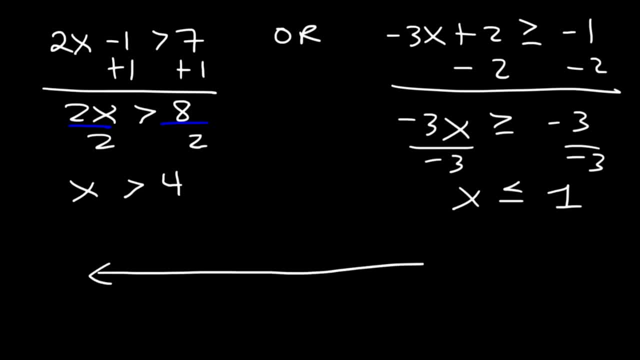 of the inequality sign. so this is the first one. this is what we have. so there's a 1. actually let's put 0. first is 0, 1, 2, 3 and then 4. so X is greater than 4, but not equal to 4. so we're going to have 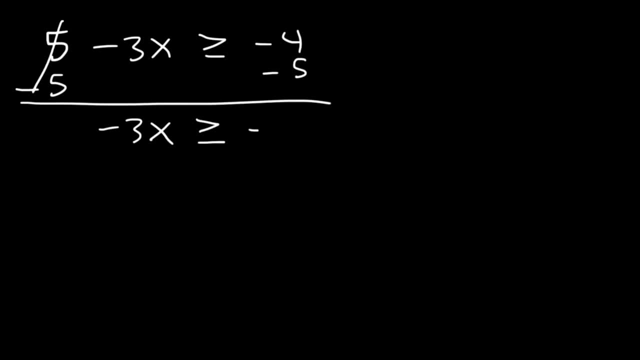 Negative 3x will be equal to or greater than negative 4 minus 5,, which is negative 9.. Next, we need to divide both sides by negative 3.. Now here's a question for you: When you divide or multiply by a negative number, does anything special happen? 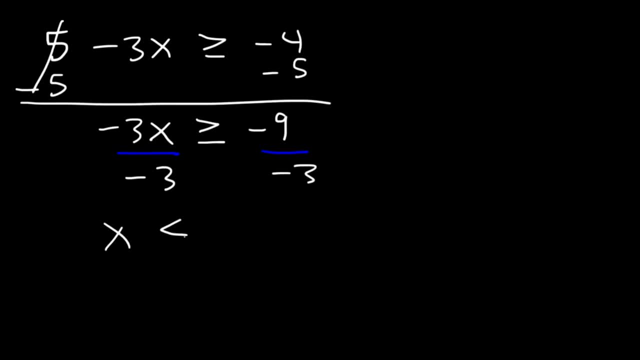 And the answer is yes. When you multiply or divide by a negative number, you need to change the direction of the inequality sign. Negative 9 divided by negative 3 is positive 3.. And now we can plot the solution on a number line. 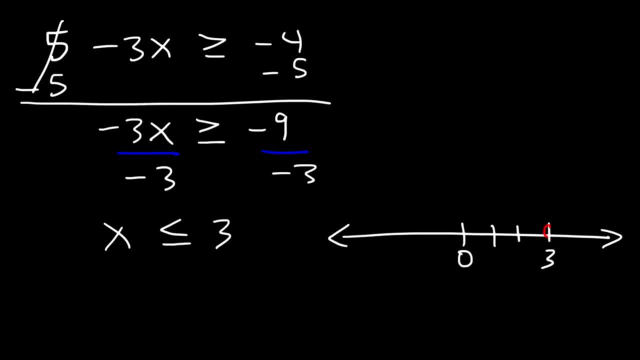 So x is less than or equal to 3.. So we're going to have a closed circle shaded towards the left because it's less than So the solution using interval notation is infinity to 3, using brackets. here's the next one. let's say: if we have 2x minus, 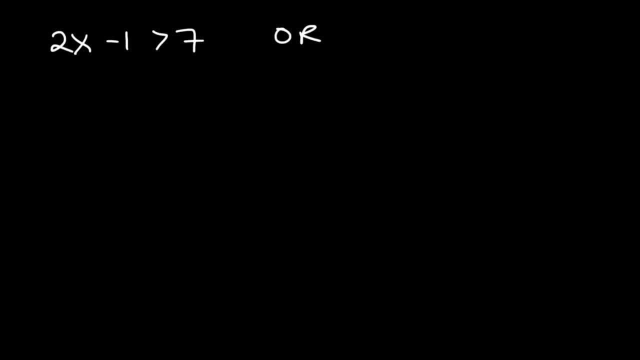 1 is greater than 7 or negative. 3x plus 2 is equal to a greater than negative 1. solve the equations. so let's start with the first one. let's add 1 to both sides, so 2x is greater than 8. next let's divide both sides by 2. 8 divided by 2 is: 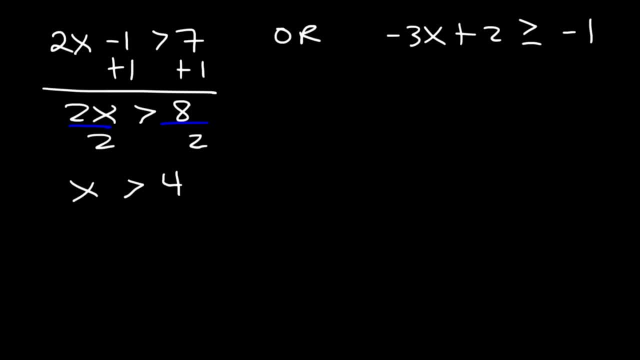 4. so X is greater than 4. now, before we plot on the number line, let's solve the other one. let's subtract both sides by 2. negative 1 minus 2 is negative 3. next, let's divide by negative 3. don't forget to change the direction of the. 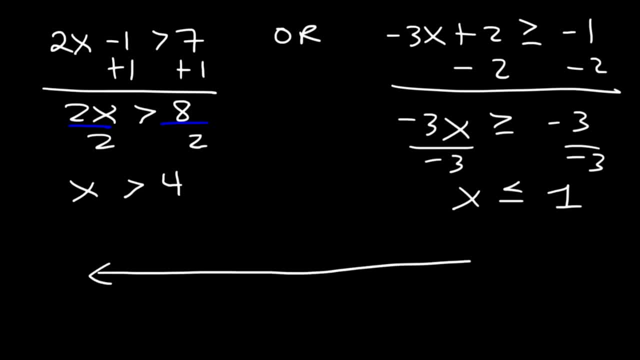 inequality sign. so this is what we have, you. so there's a 1. actually let's put 0. first is 0, 1, 2, 3 and then 4. so X is greater than 4, but not equal to 4. so we're gonna have an open circle at 4. 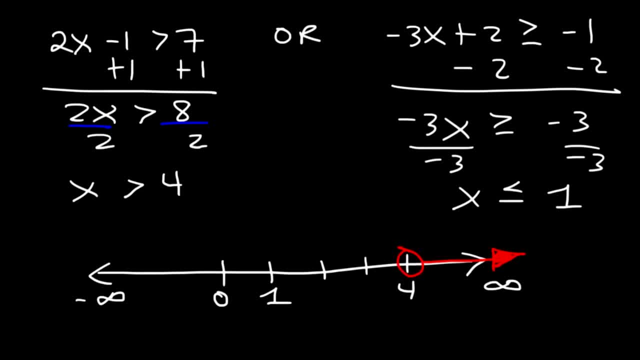 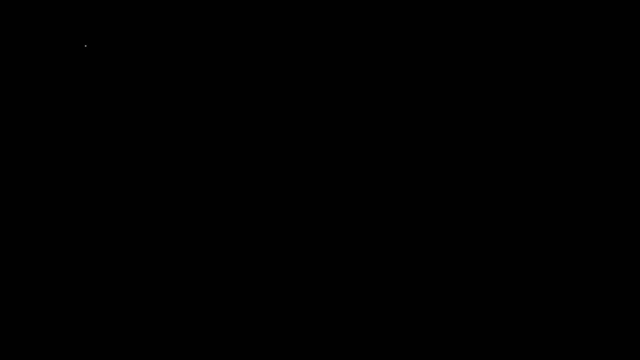 shaded towards the right. now, X is less than or equal to 1, so we're gonna have a closed circle shaded towards the left, since it's less than 1. so using interval notation, the answer is negative infinity. so, won using brackets, union 4 to infinity. and that's it. let's try one more example. let's say: 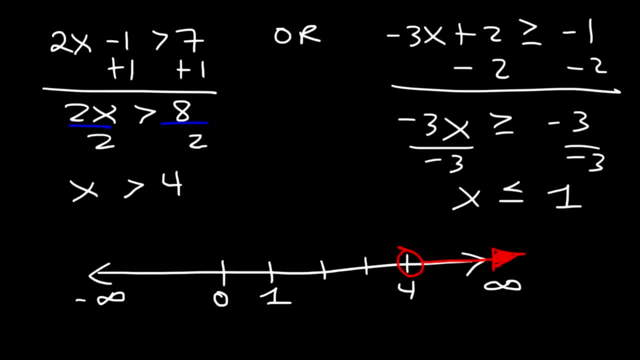 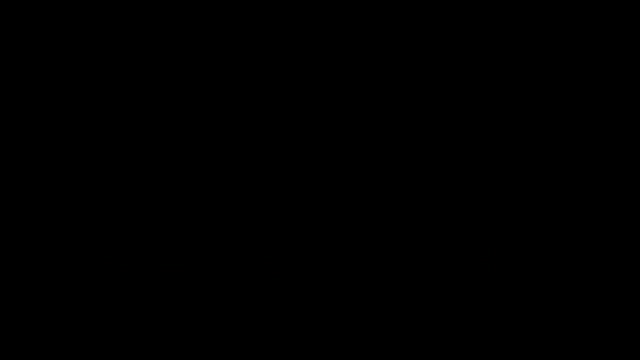 an open circle at 4, shaded towards the right. now, X is less than or equal to 1, so we're going to have a closed circle shaded towards the left, since it's less than so. using interval notation, the answer is negative: infinity to 1. using brackets, union 4 to infinity. and that's it. let's try one. 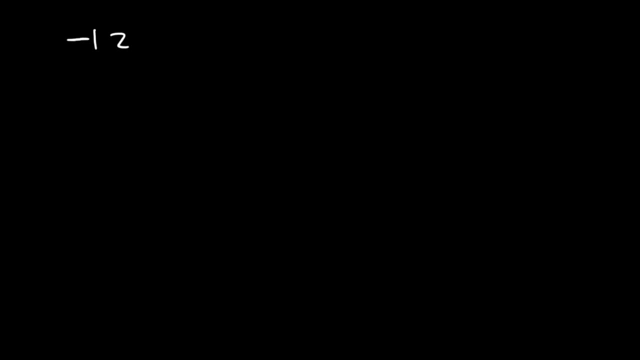 more example. let's say negative 12 is less than 7. X minus 5, which is less than or equal to 9. find a solution. so here we have a compound inequality with three sides to an equation. So let's add 5 to all three sides. Negative 12 plus 5 is negative 7.. 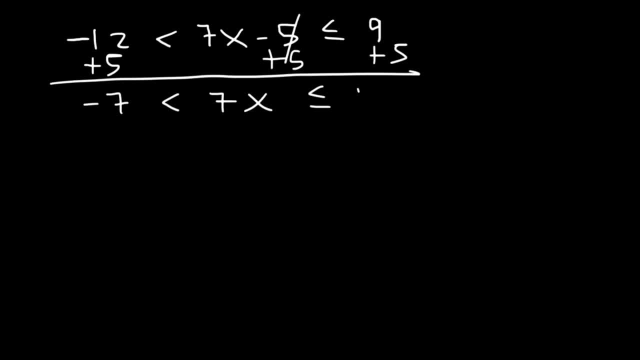 Negative: 5 plus 5 is 0.. 9 plus 5 is 14.. Next, let's divide each side by 7.. Negative: 7 divided by 7 is negative 1.. 7x divided by 7 is just x. 14 divided by 7 is 2.. 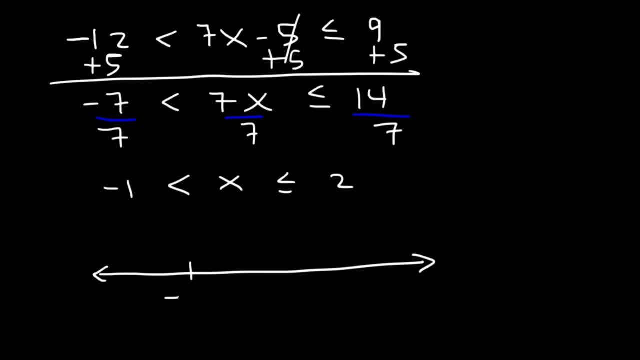 So x is between negative 1 and 2.. x is greater than 1, but not equal to it, so we're going to have an open circle shaded towards the right. x is less than or equal to 2, so we're going to have 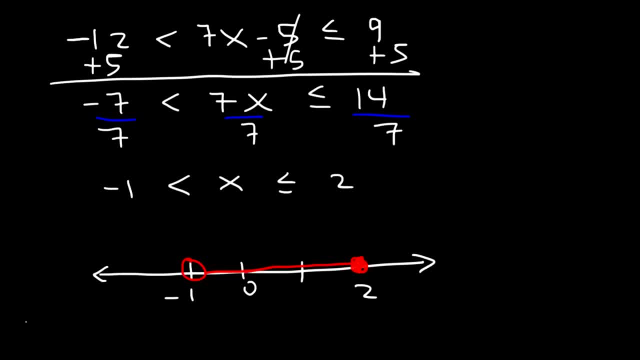 a closed circle shaded towards the left, so it's between these two values. So an interval notation is from negative infinity to 2.. So you have a bracket which is associated with the closed circle and a parenthesis that is associated with the open circle. Thank you. 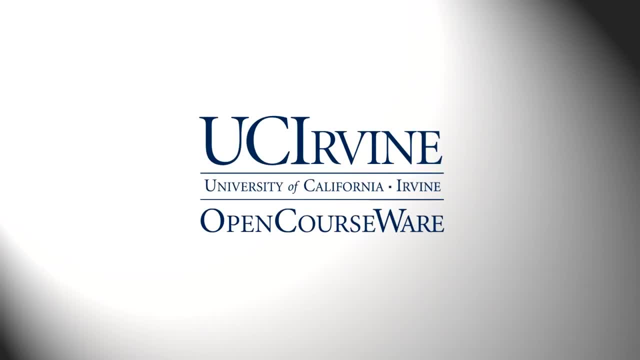 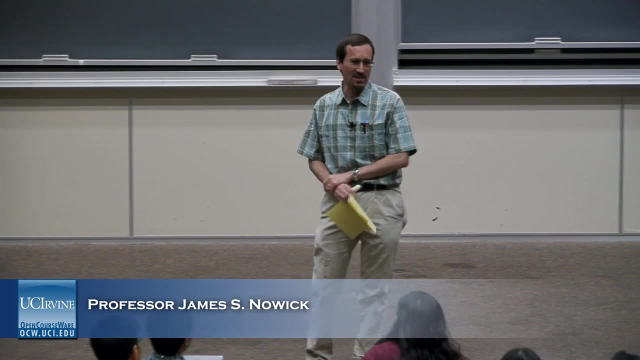 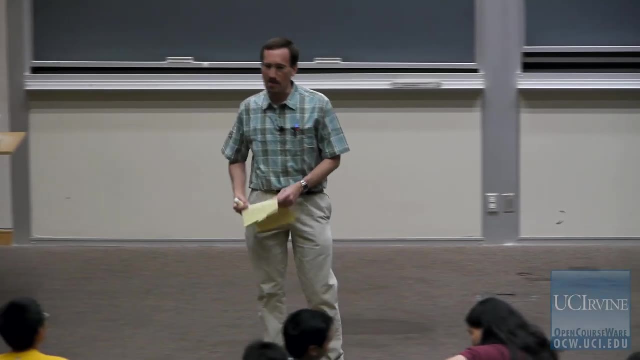 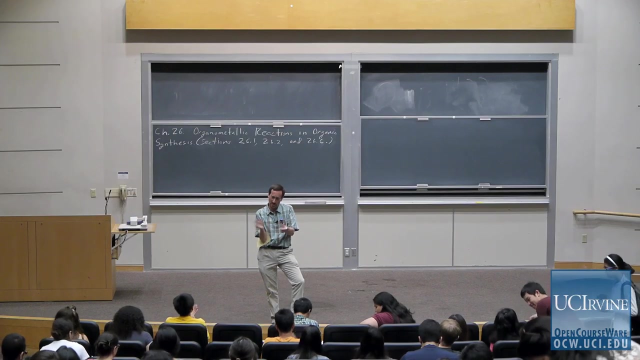 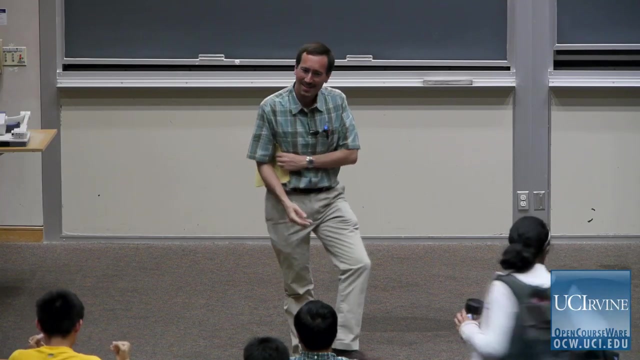 Good morning. Good morning, Oh. this feels good today. This feels like we are at the end of a very long journey and we've learned so much, And I wanted to start by thanking you for coming along with me on this journey.